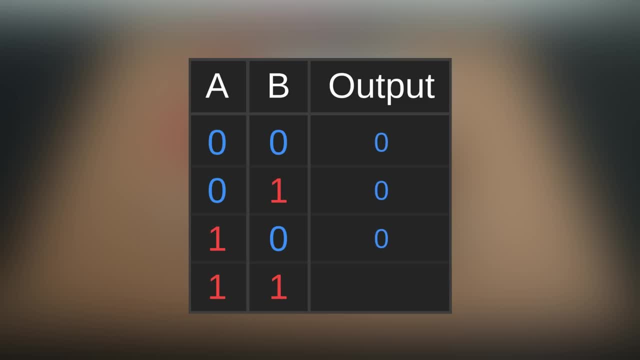 configurations we could have. And here's the output: 0, meaning the light would be off, and 1 meaning it'd be on. Since that's only the case when A and B are one, this is known as the logical AND operation, And this kind of table, by the way, is called a truth table. 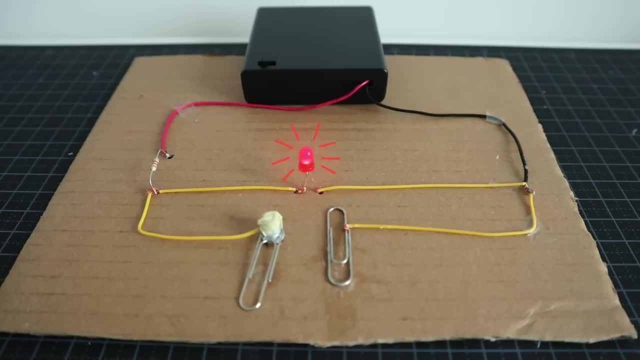 Here's a bit of a different circuit. this time we only have one switch and even though it's open, the light is currently on. If I close the switch now, the light will go off, because we've created an easier path for the current to travel. so we're essentially 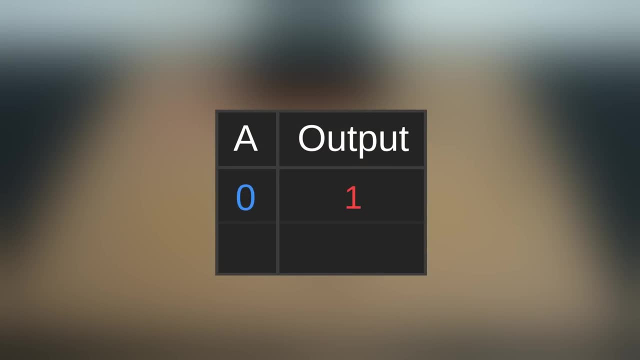 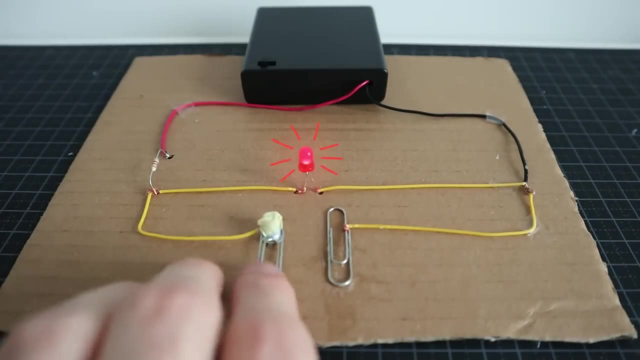 inverting the input. If the state of the switch is 0,, the output is 1, and vice versa, and this is known as the logical NOT operation. Now I've been controlling these switches with my fingers, which computers sadly lack. 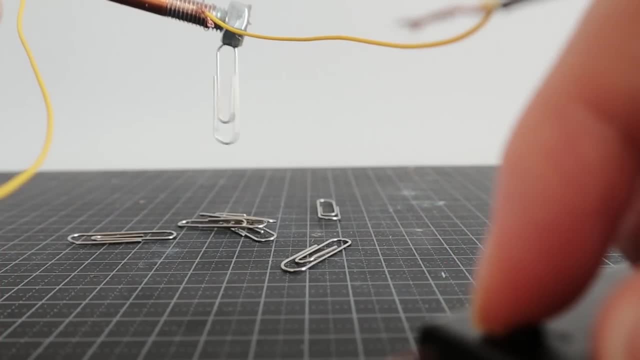 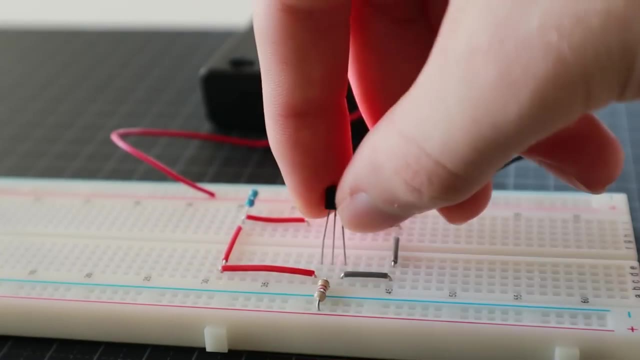 in the very early days electromagnets were used to open and close the switches, but this was kinda clunky and slow. so then came fancier technologies like vacuum tubes and finally transistors. As a tiny example of what transistors do, this is essentially that same. NOT thing from. 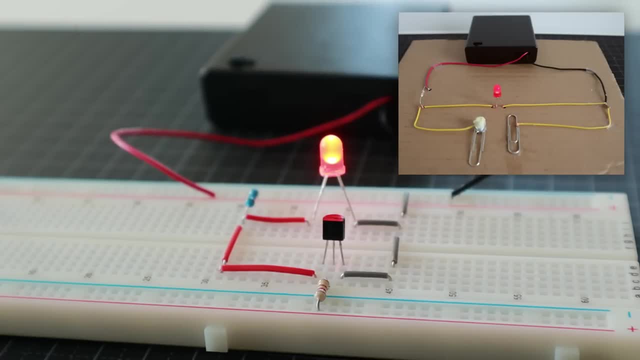 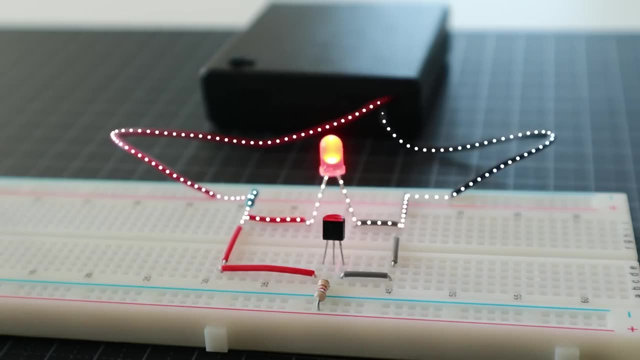 before, just set up on a breadboard and with a transistor in the place of the paperclip switch. If we think of the current flowing in this circuit, it would look something like this: It can't flow through the transistor at the moment because right now it's acting. 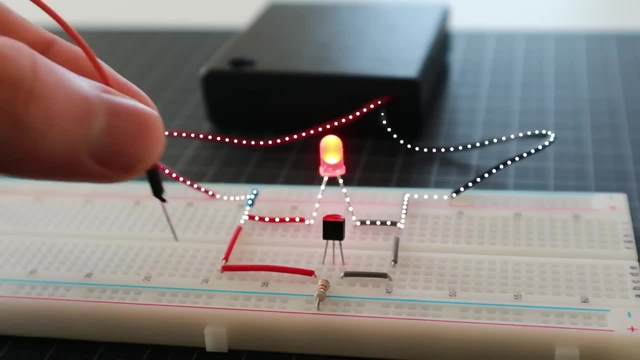 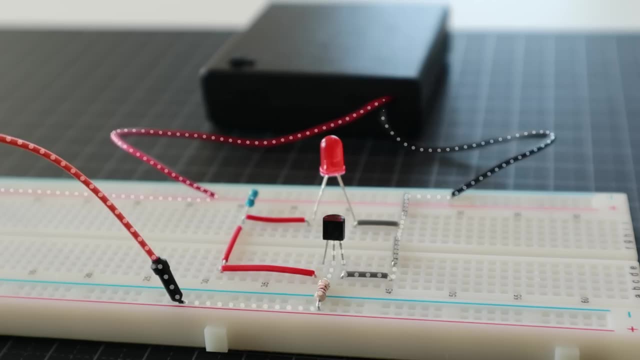 as an open switch. But if we send power to the middle pin of the transistor, establishing a small flow of current like this, the fancy physics of the transistor will make it act like a closed switch instead, allowing the main current to flow through it like so Just. 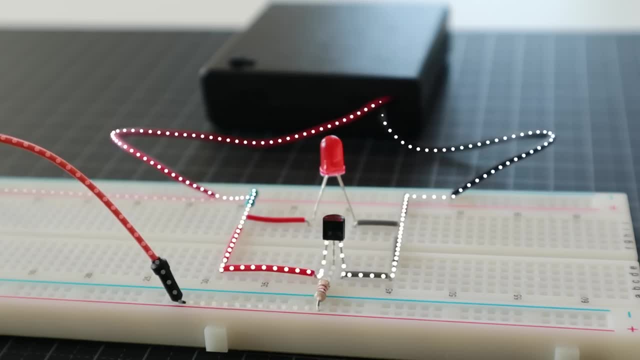 like before the light is turned off, because we've created a much easier path for the current to take. So essentially, the transistor is a switch which we can open and close with electricity instead of our fingers. I'd love to one day try and build a simple computer. 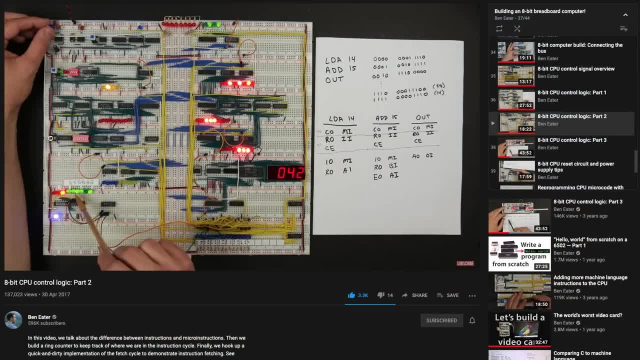 out of components like this, which is what Ben Eater has done in his very cool 8-bit breadboard computer series. but that's a little intimidating for me at the moment. so instead I've made a simplified and abstracted little simulation where we have our two logical building blocks. 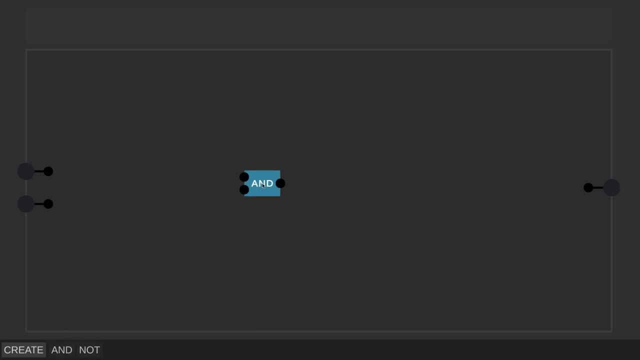 and a NOT, and we can play around and try to figure some stuff out. So on the left, here are some inputs which can be turned on and off, or we can also think of it as true and false, or one and zero. it doesn't really matter. 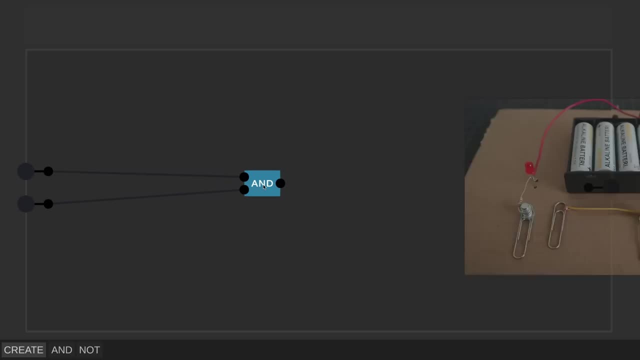 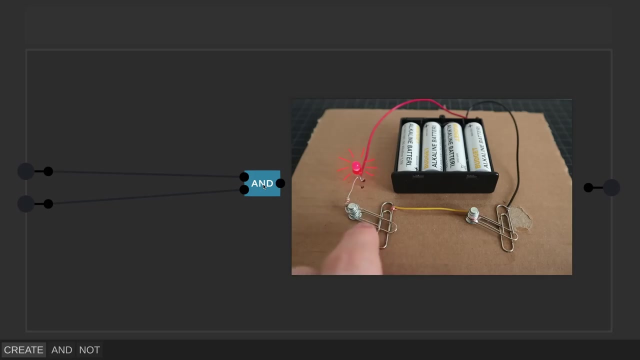 But I'll wire these up to the inputs of the AND gate and, if you recall my sophisticated circuitry from earlier, the two inputs simply control whether these switches are open or closed, which should be achieved using transistors, not paperclips, of course. 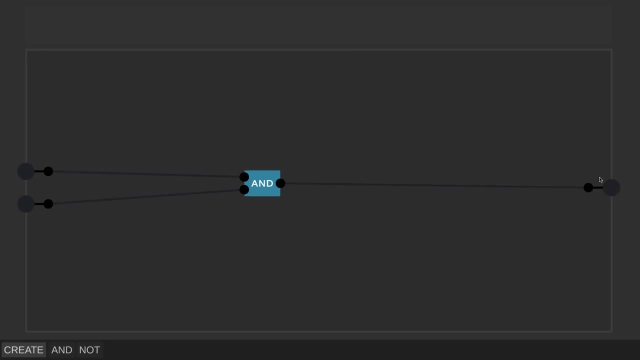 Now I'll connect the result of this AND gate up to my output node over here, and so this will only light up if both inputs are on. Let's get the NOT gate participating as well. so I'll connect it up over here and wire. 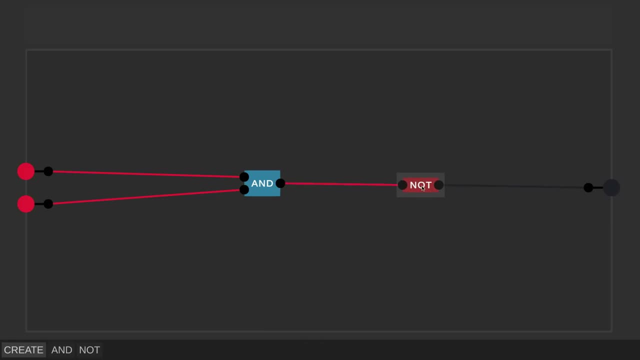 the result of that to the output instead. So the output is now inverted: it's off when both inputs are on, but in all other cases it's on. Here's a truth table for this thing we've just built, and it actually has a name: this: 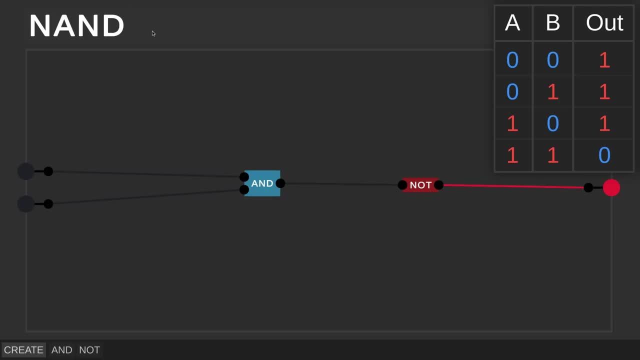 is the NOT AND or rather NAND gate. If I click on the create button down here, it'll package that up into its own little chip and we now have a NAND gate to mess about with. I guess this is a good moment to mention NAND2Tetris, which, along with Ben's videos, is a fantastic 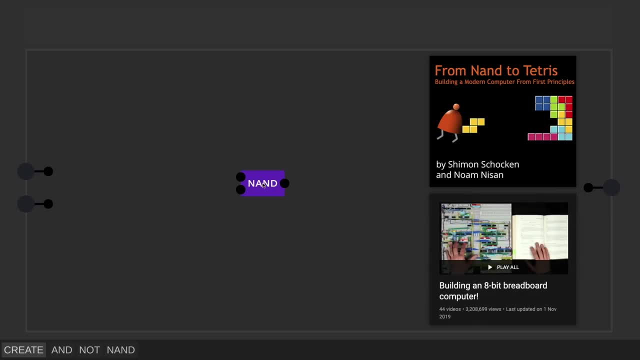 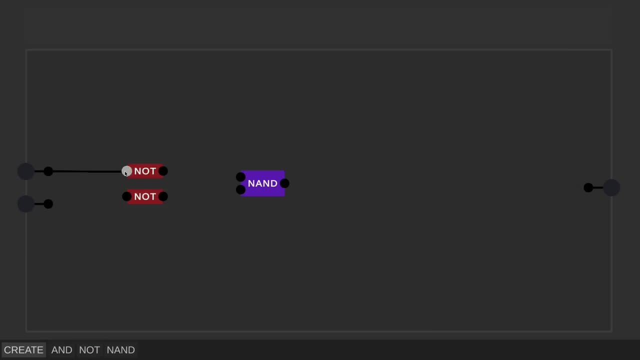 free resource I've been using to learn more about this stuff, so I recommend checking that out if you're interested. Anyway, to take this a little further, we could maybe try inverting both of the inputs before feeding them into the NAND gate and let's see what that does. 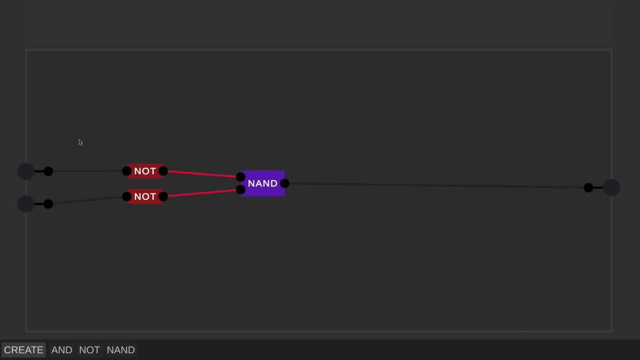 So with both inputs off, the output is off. if I turn either of them on, the output goes on, and if both are on, the output is still on. So we've created what's called an OR gate and I'll turn that into its own little chip. 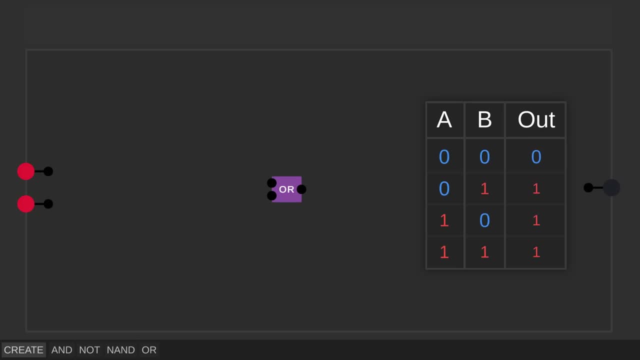 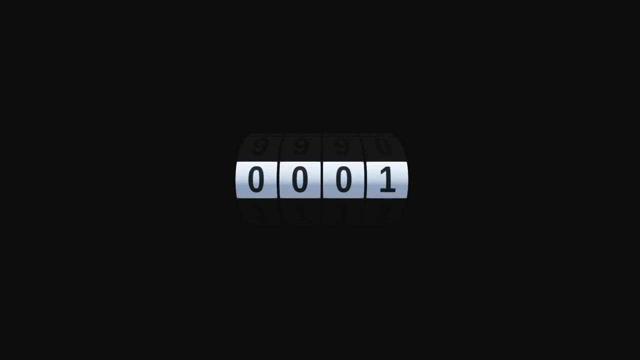 as well. This seems pretty useful, And here's the truth table for that. Alright, let's take a moment to think about something that's pretty important to computers – numbers. In the decimal system that we know and love, there are 10 digits, 0 through 9, and if we 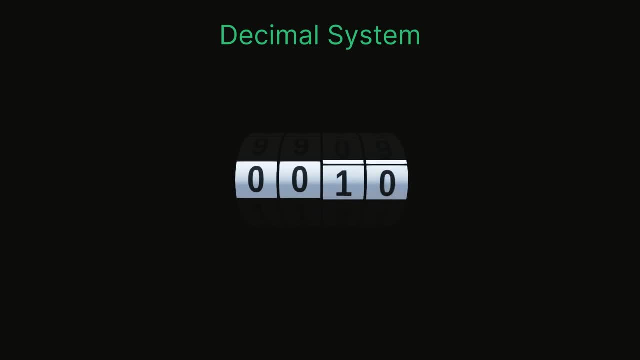 want to go higher than that, we need to add another place to the left where each digit actually represents 10 times as much as those in the previous spot, and we can have as many places as we need. so here would be hundreds, then thousands, and so on. 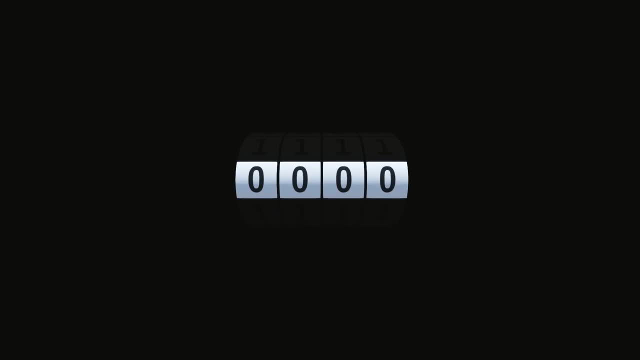 In the realm of electronics, though, it's easier to work with just two digits, because they can be naturally represented with a low voltage or a high voltage, So this binary system works in the exact same way as the decimal system. it's just that. 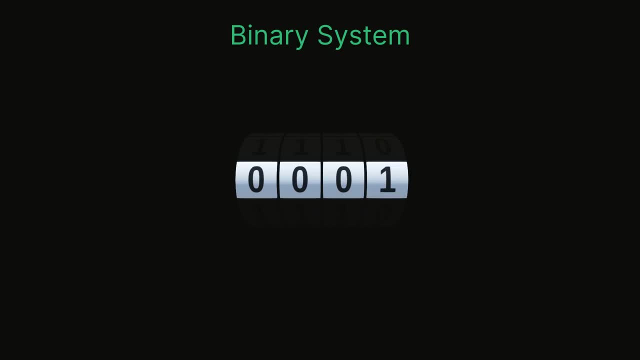 once we reach one, we've already run out of digits, and so we increment the place to the left. Because there are only two digits in binary, each place is worth two times more than the last. First place is worth 1,, then this place is worth 2, then 4, then 8, and so on. 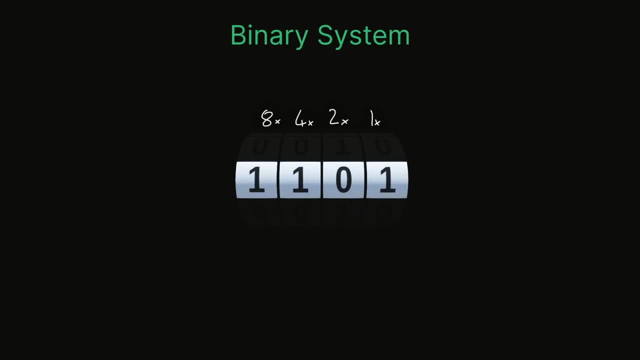 So let's say we want to figure out what this sequence- 1101, would be in decimal. Well, we can write it out as 8 times 1, plus 4 times 1, plus 2 times 0, plus 1 times 1,. 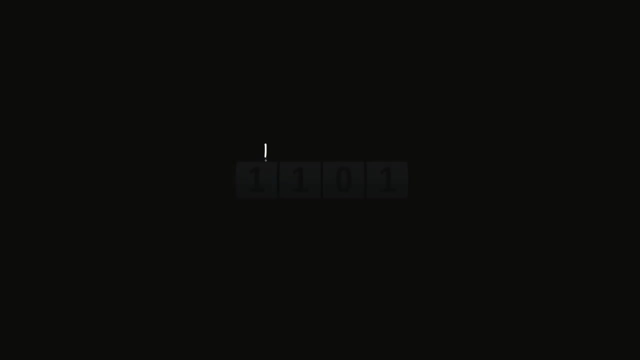 and that comes out to 13.. Alright, now what I'd like to do is design something that's able to add two binary numbers together. So let's work through a quick example by hand. Say we want to add these two numbers Starting on the right here: 1 plus 1 is 2, which in binary, is 10.. 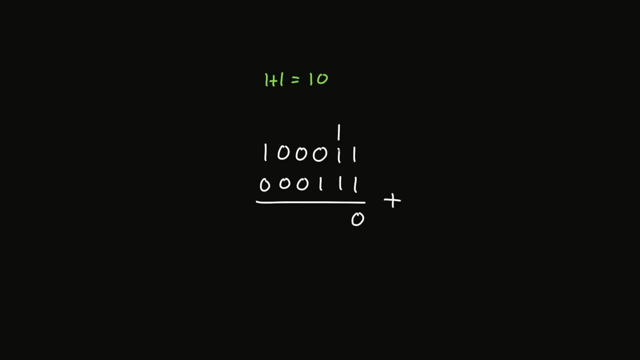 So I'll write the 0 down here and then carry the 1 over up here, because we'll need to add it together with these other two in order to figure out what goes in this spot. By the way, this part that we wrote down here straight away I'll refer to as the sum bit. 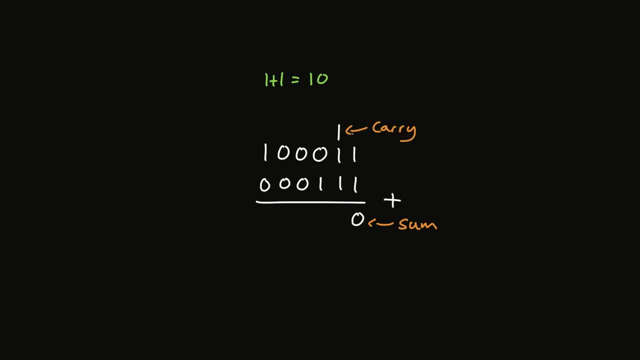 and this one up here is the carry bit. Okay, let's continue. 1 plus 1 is 2, plus the carry gives us 3 in decimal or 11 in decimal. So let's write the sum down here and then carry the 1 over up here, because we'll need. to add it together with these other two in order to figure out what goes in this spot. If we like, we can write the sum down there and then carry the 1 over up here, because we'll need to add it together with these other two in order to figure out what goes in this. 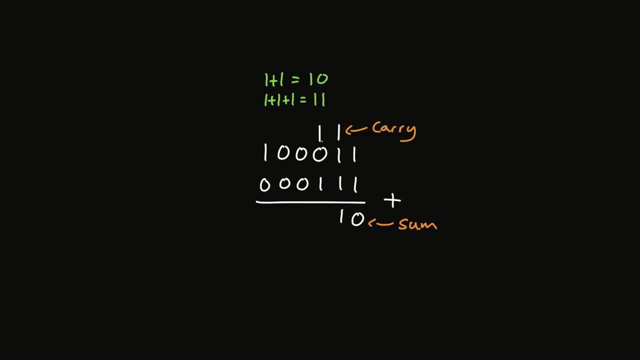 spot. So 1 plus 1 is 2, plus the carry gives us 3 in decimal or 11 in decimal. So I'll write 1 over here- that's the sum bit- and carry the other one over to the left. 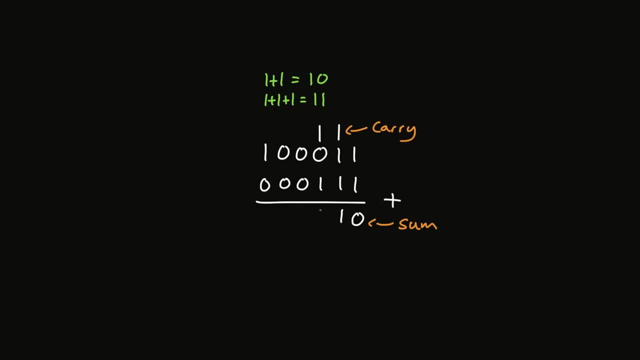 Now we have 0 plus 1, plus the carry bit is 2 again, So I'll put 0 down here and 1 up here. This will just give us 1, so I'll write that down here. Then 0 plus 0 is 0. 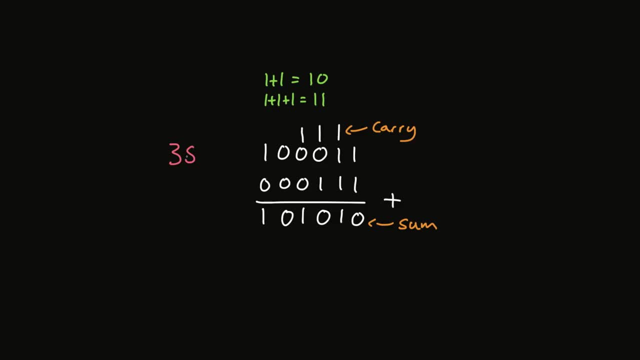 And finally, 1 plus 0 is 1.. In case you care to know, what we've just calculated here is 35 plus 7.. It's a little daunting to track in a decimal. start thinking about how we can wire our logic gates together to do all of this. So let's start. 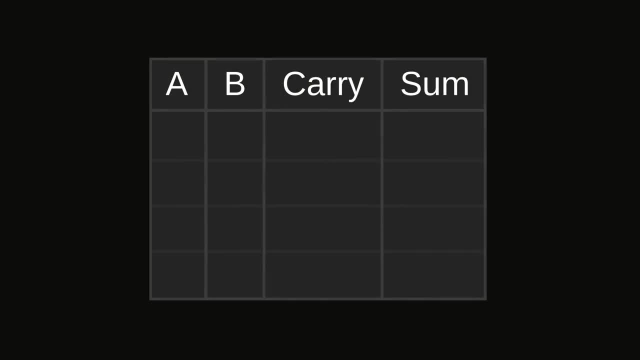 small with adding together just two single bits. For example, if we're adding a zero and a zero together, then naturally both the carry bit and the sum bit will be zero. But if the first bit is a zero and the second is one or the other way around, then the carry bit will be zero and 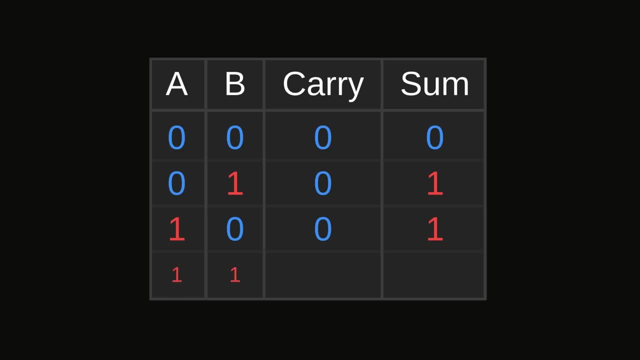 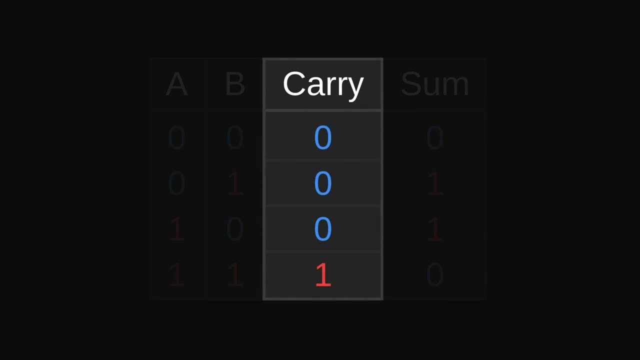 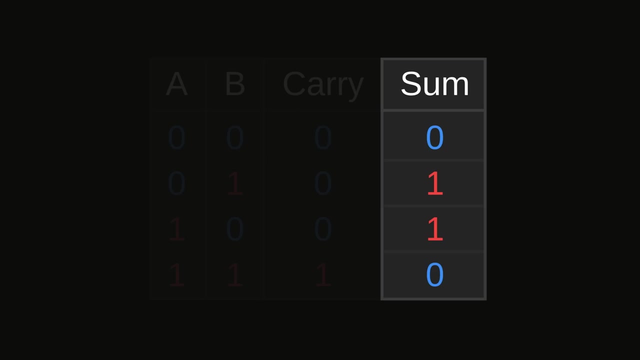 the sum bit will be one. Finally, if both bits are one, then the carry will be one and the sum bit will be zero. So if we look at the carry column here, it might look familiar, because it's actually an exact match with the AND operation. The sum column, on the other hand, doesn't match. 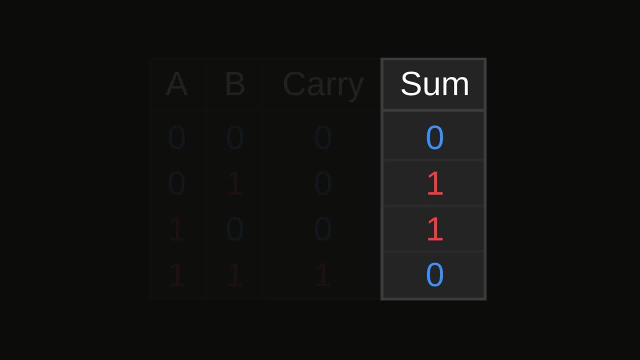 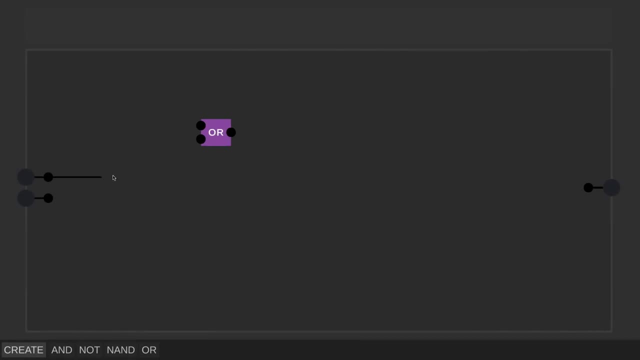 exactly with anything we've already seen, But it's quite close to the OR gate we created earlier. it just has a zero in this last spot instead of a one. So let's take that OR gate as a starting point And we just need to turn the output to a zero when both inputs are one. So I'm going to 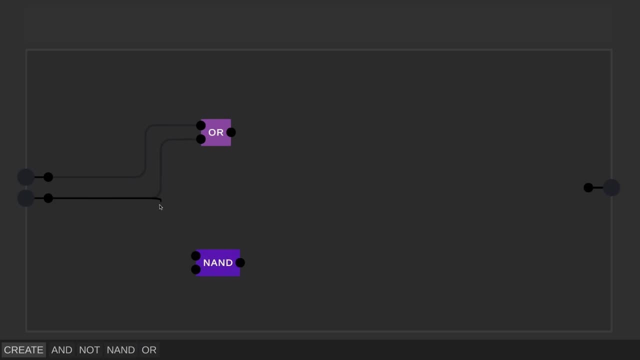 take a NAND gate and connect it to the OR gate, And then I'm going to take a NAND gate and connect it up here And this will check if both inputs are one and then invert the results that it's outputting zero in that case. We can then use an AND gate to check if either of the inputs is one. 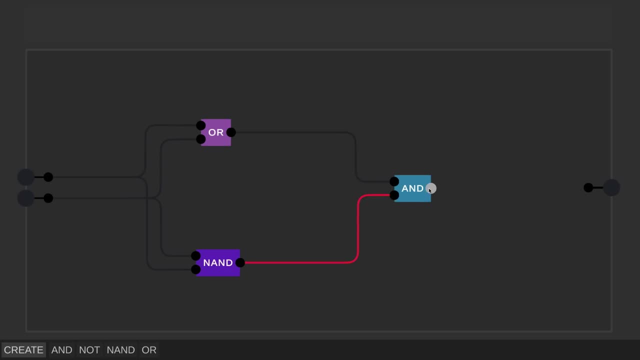 but not both of them. Let's test this quickly: With both inputs, off or zero, the output is zero. With just a single input set to one, the output is one, But, crucially, when both inputs are one, the output will be zero again. This operation has a special name as well. 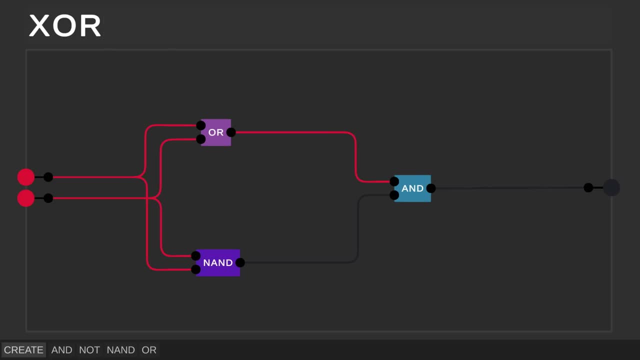 it's called an exclusive, OR XOR for short. Okay, so I now have an empty chip with two inputs which we want to add together and two outputs, the sum bit and the carry bit, So we can use our new XOR gate to calculate the. 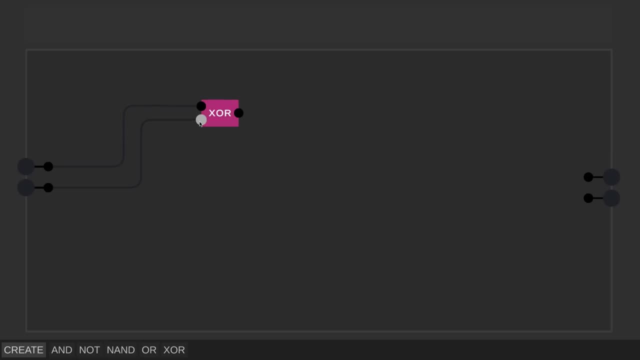 sum bit of the two inputs, And then remember that only if both inputs are one should the carry bit be one, And so we can simply use an AND gate to test for that. So that's everything. we need to add two bits together, But of course. 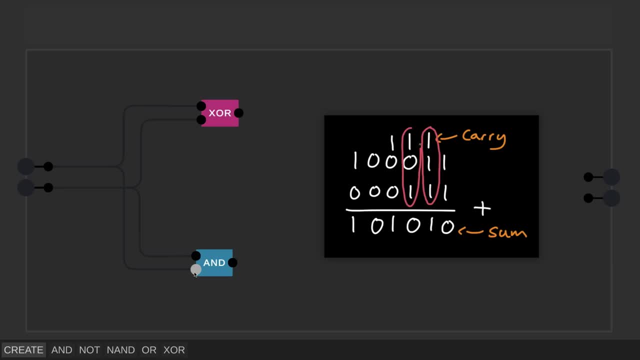 in some of the steps we actually had three bits we needed to add together because there was a carry bit from the previous step to deal with And in fact we could think of these other places as having zero in the carry spot. So in a way, we're always adding three bits together. 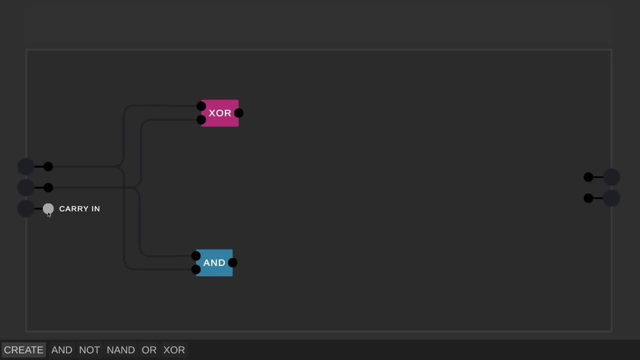 So I'll introduce a third input to the chip over here for the carry input, And we need to add this to the sum of the first two bits which we calculated up here. To do that we can simply use another XOR gate wired up to that carry input. 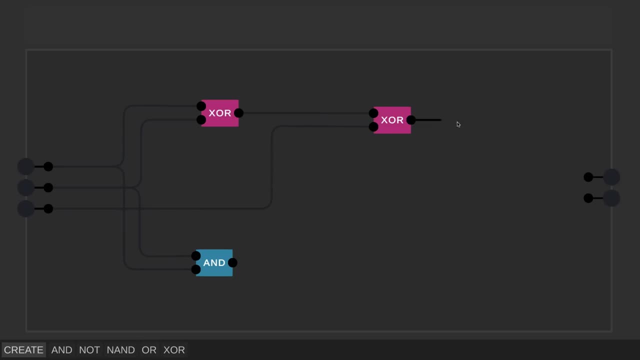 and to the sum of the first two inputs. We'll then need a second AND gate as well, because if the sum of the first two bits is one and the carry input is one, then we'll need to carry one to the next step. 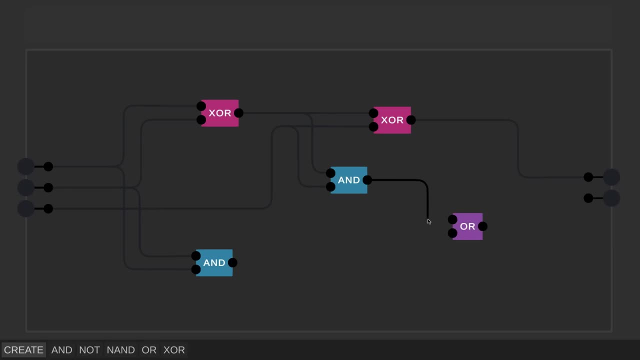 So if either of our two AND gates detect that we should be carrying one, then we'll of course want to output one to the carry output, which we can do using an OR gate. Let's check if this is working properly. So, with all of the inputs off or zero. 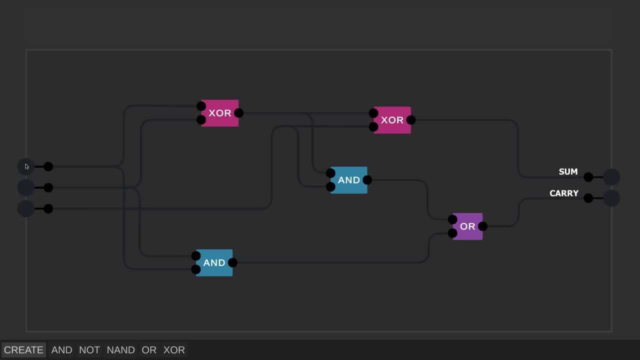 both the sum and the carry output bits should be zero. Then if any single input is one, the sum should be one and the carry should be zero. So far, so good. Next, if any two inputs are one, then the sum bit should be zero and the carry should be one. 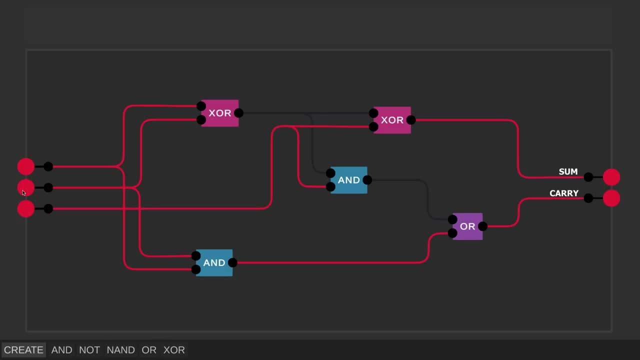 And finally, if all three inputs are one, then the sum should be one and the carry should be one, And it looks like it's all working, so I'll give it a name. And then what I'd like to do is take this adder we've made and use it to construct a 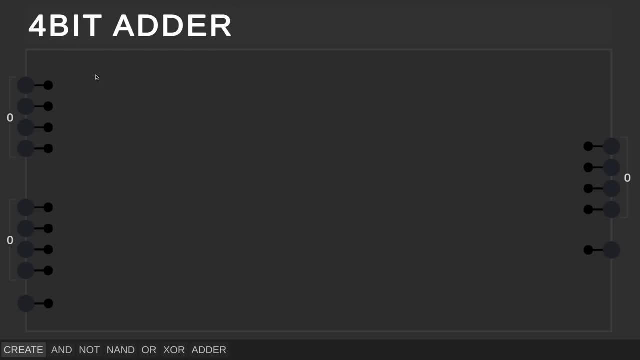 4-bit adder capable of taking these two 4-bit numbers that we have as our inputs and calculating the 4-bit sum as the output. I've added these little displays, by the way, to tell us what all these values are in decimal. 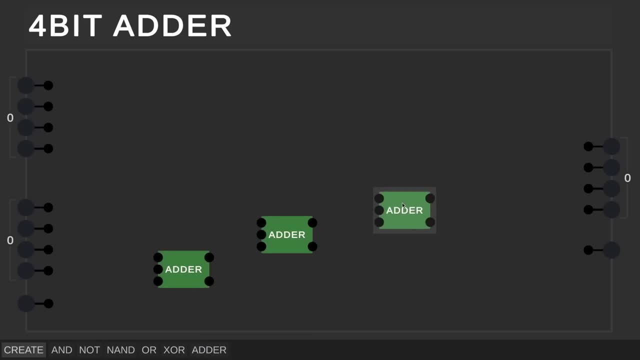 just so it's a bit easier to tell if this thing is working. So we'll need four adders to construct this and I'll wire each one up to the outputs. There's a carry input here, just in case we want to string two 4-bit adders together. 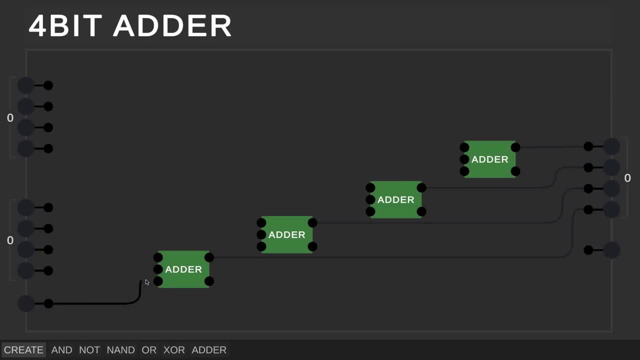 to make an 8-bit adder, for example, go into the carry input of the first adder and then its carry output goes into the carry input of the next one, and so on down the chain. Finally, I need to connect up the two 4-bit inputs. 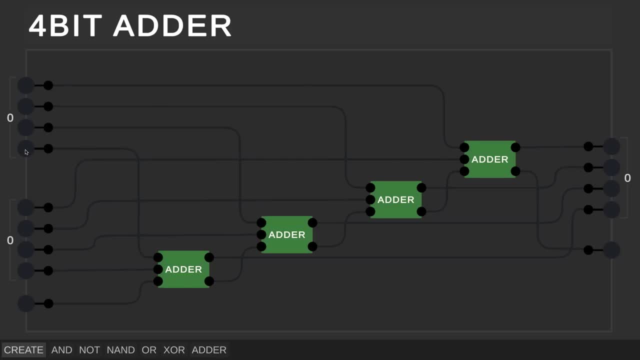 Let's test this out. So right now we have: 0 plus 0 equals 0,, which is a good sign. Let me try: 1 plus 1,. 2 is correct, 5 plus 1 is 6, and 7 plus 1 is 8,, so it looks like we can add numbers. 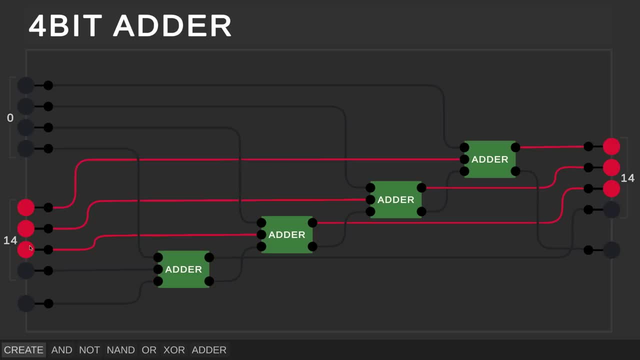 together, which is pretty cool, Of course, with just 4 bits. if we try to do 15 plus 1, for example, it will overflow to 0, because we don't have enough bits to store 16, and the carry bit will light up over here telling us the result was too big for 4 bits. 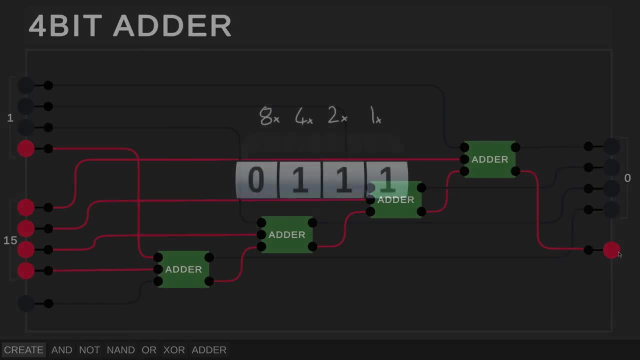 If we want to extend this to handle subtraction, we'll need a way to represent negative 1 and negative 2.. If we want to extend this to handle subtraction, we'll need a way to represent negative numbers in binary. I always assumed that this last spot was used to indicate 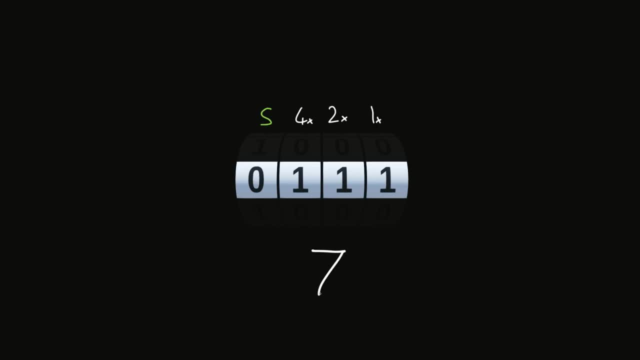 the sign of the number. so what we have here would be positive 7, and this would be negative 7.. But of course you'd expect that if we added 7 to negative 7, we'd end up with 0,, but that's. 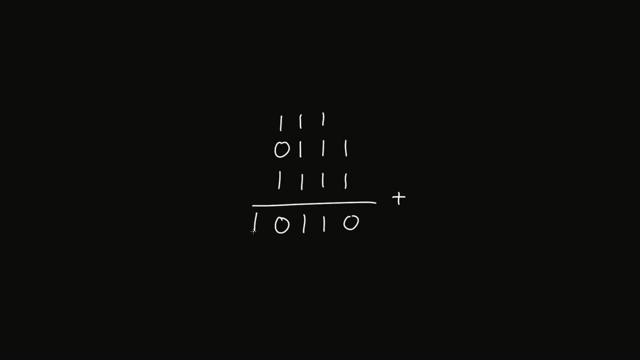 clearly not the case here. So one way we could try thinking about this is: what would we have to add to 7 in order to get 0 as the result? Well, in order to get a 0 in the first spot, we'd need a 1, because, remember, 1 plus 1 gives us a sumbit of 0.. Of course, we also now have to. 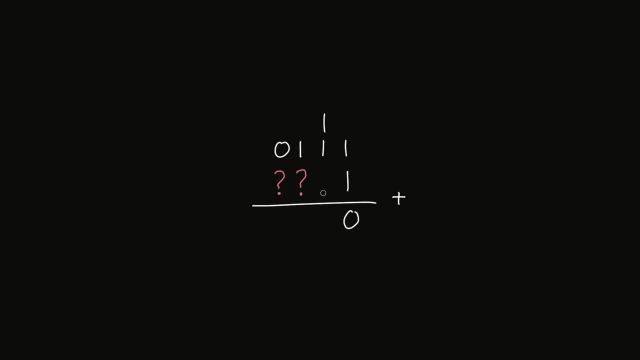 carry 1 to the next spot. So now we know that there should be a 0 here, so that we'll again have 1 plus 1, giving us a 0 for our sumbit and a carry of 1.. We can then deduce that there should: 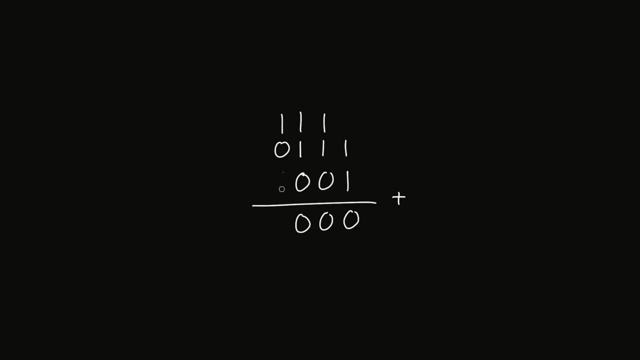 be a 0 here as well, and we can continue like this to end up with all 0s for our 4 bits. There is a 1 that ends up over here, but since we're working with just 4 bits, that can be. 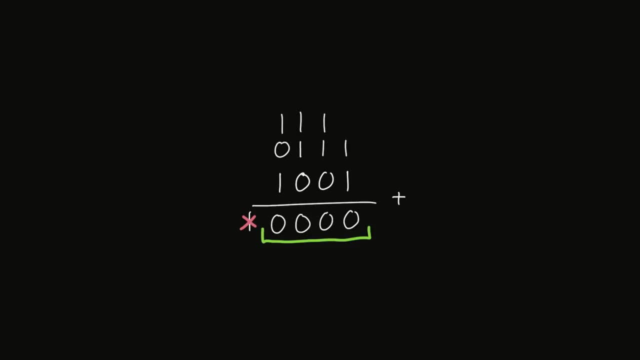 discarded. So we've figured out that negative 7 must be 1001.. That might seem a bit weird, but it actually makes some sense if we think of this last spot as the negative 8 place, because then we could write this out as negative 8 times 1 plus 4 times 0 plus 2 times 0 plus 1. 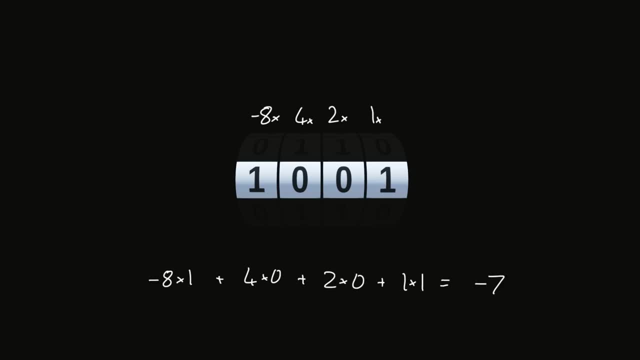 times 1,, which gives us negative 7.. Let's start at 0, and see what it looks like now. if we count up, So 7 is now the largest number we can have with 4 bits, and it then flips over to the smallest number, negative 8.. And from there we have negative 7,. 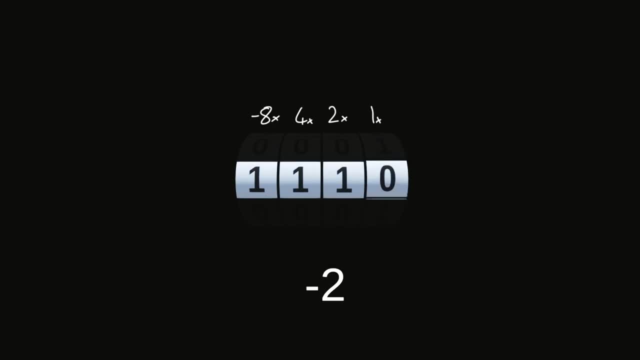 negative 6,, negative 5, negative 4,, negative 3,, negative 2, and finally, all 1s would be negative 1.. So it's a bit of a funky system, but it allows us to add negative and positive numbers together. 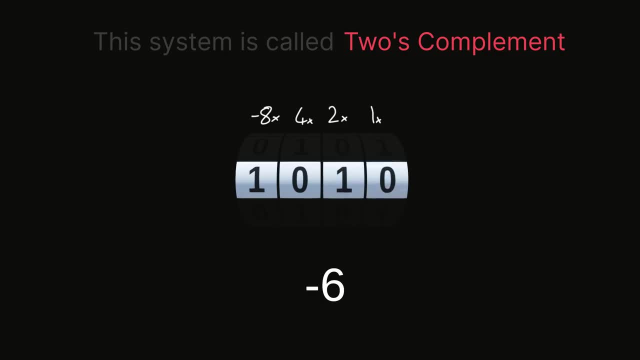 without any fuss. so it's totally worth the weirdness. Now there's actually a simple two step process for getting any positive number negative. Take the number positive 6, for example, 0110 in binary. The first step is to invert all the bits, so where there's a 0, we write a 1,. 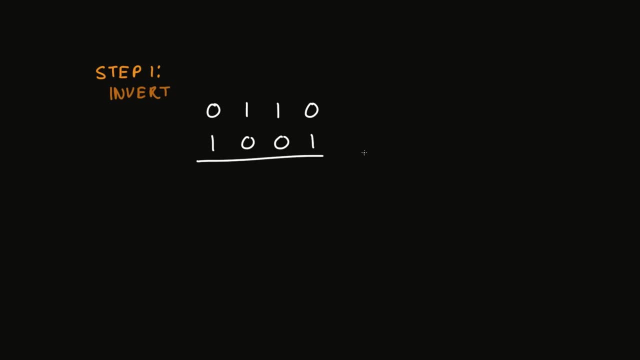 and vice versa, giving us 1001.. At this point, if we were to add these two together, we'd obviously get all 1s. We want it to be all 0s, though, and we saw a few minutes ago that if 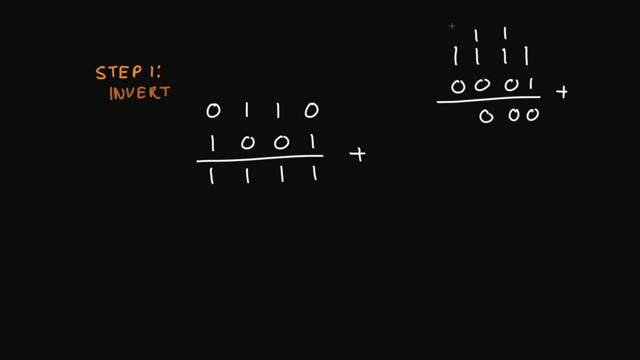 we take this and just add 1 to it, we'll end up with 0 for the 4 bits we're interested in. This tells us that clearly our inverted number is just 1 too little to give us all 0s. so the second step, as you might predict, is to take the inverted number and just add 1 to it. 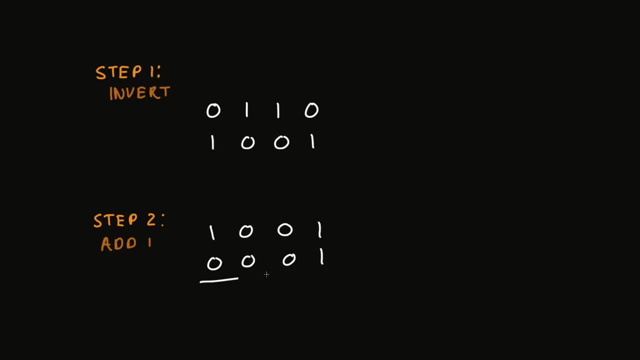 So in this case we'd take 1001 and add 1, and that would give us 1010. And if we look back at the number wheel, that is indeed negative 6.. So using that 4-bit adder we built, we can of course add these two 4-bit numbers together. 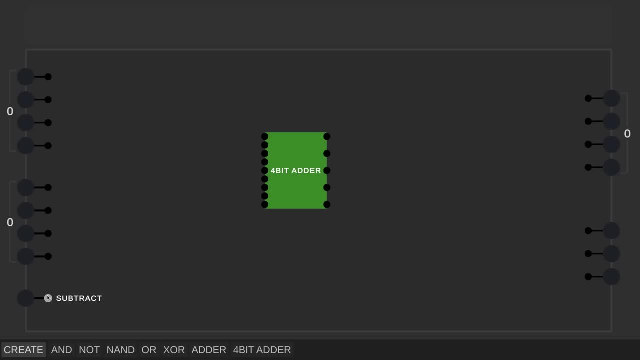 and we can also invert them. So if the subtract signal over here is on, then I want to subtract the second number from the first, which we can do by making the second number negative, and remember, we do that by inverting the bits and then adding 1.. So to invert the bits, 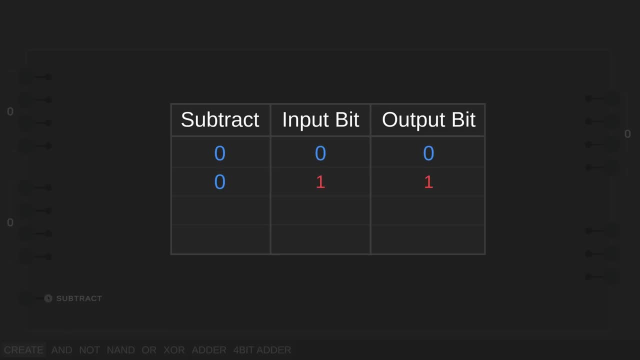 we need something that looks at the subtract signal, and if that's off, the input bits should be unchanged, but if the subtract signal is on, then the bit should be inverted Conveniently. this table actually matches the exclusive OR we made earlier. 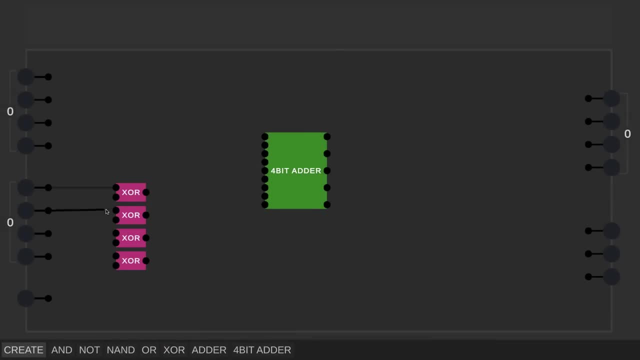 so we can invert these bits only if the subtract signal is on. The last step of negating a number was to add one, so we can just feed the subtract signal into the carry input of the adder and that'll do that for us, Alright. 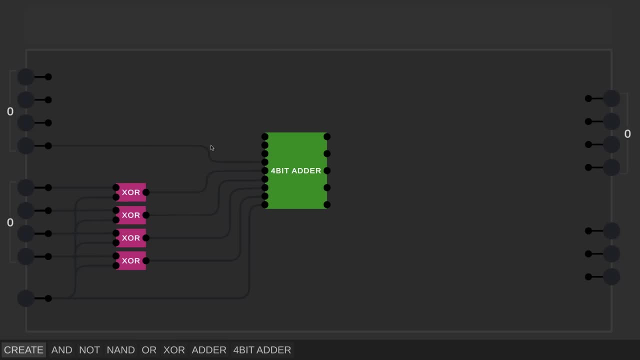 I'll quickly go ahead and wire up the rest of the inputs and then output the result. I also have these three extra outputs, and these are just for flagging some stuff about the result. This one over here, for example, tells us if the result was 0, and we can test for that, like so. 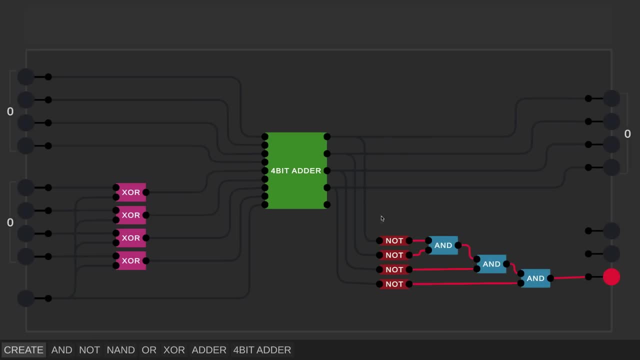 This other output tells us if the result was negative, which is true if our negative 8 bit is set to 1.. And finally, there's the carry which I can just take from here, And this is just information that'll be useful to us later on. Let's now test if this is actually. 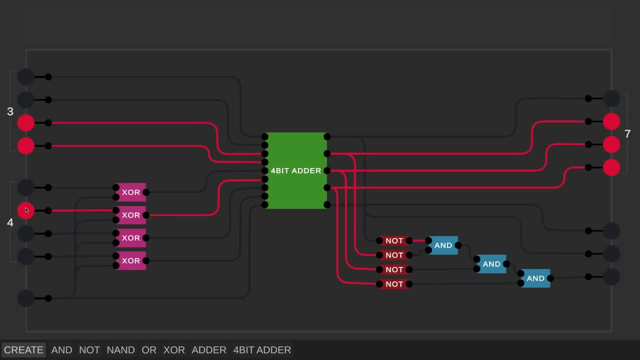 correct. So I'll try 3 plus 4, and that's 7,. so it looks like we haven't broken addition at least. Now I'll try turning on the subtract signal. so we're doing 3 plus negative 4,. 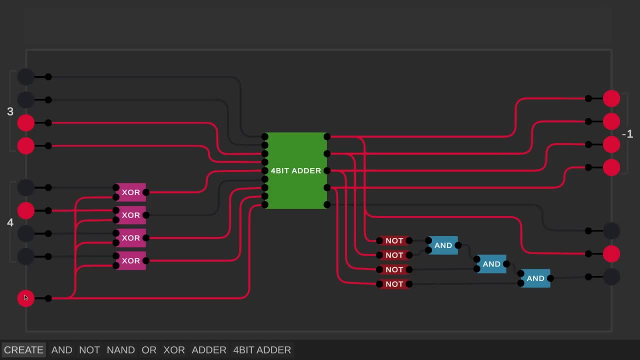 which of course is the same as saying 3 minus 4, and the result is indeed negative 1, so that's good. Let me try negative 2 minus 4, and that gives us negative 6.. Then let's see if it can handle subtracting a negative number. so I'll try negative 2. 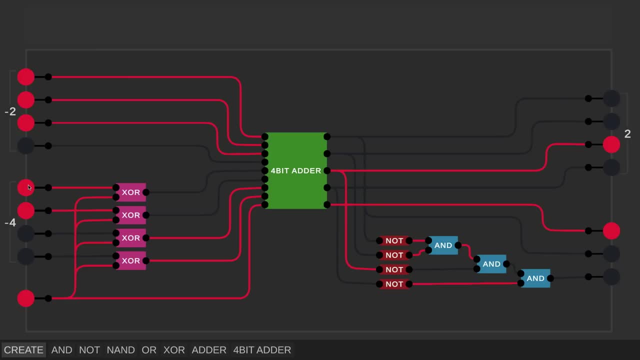 minus negative 4.. Even that seems to work, we get positive 2.. I want to test one last thing, which is adding two negative numbers together, and once again the math seems to check out. So this is going to be our arithmetic and logic unit, although to be honest, it doesn't actually. 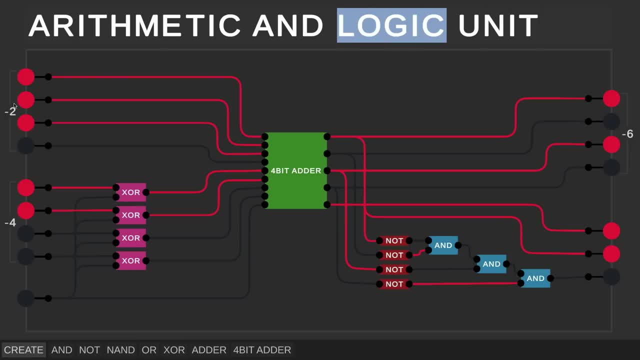 do any logic. there would just be things like doing the AND operation on the inputs and outputting that, for example. But we can expand this later if necessary. For now I'll call it ALU for short and package it up into a tiny little chip.